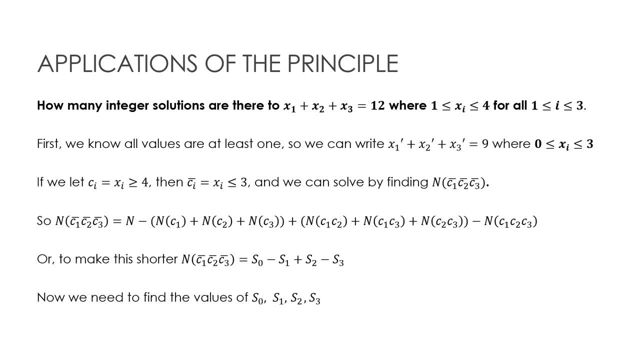 so far. Now, here's what I know. I know that all of the values are at least 1, because it tells me right here: x1 is at least 1 and at most 4.. So what I'm going to do? 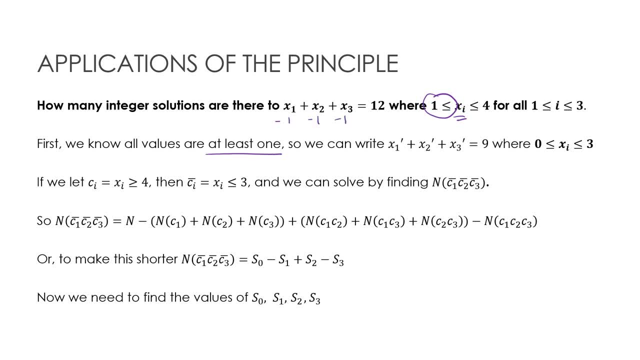 is I'm going to subtract 1 from each of those, which means that after subtracting 1, I'm going to call this x1 prime, which means it's not the x1 I started with. I've taken 1 away- x2 prime. 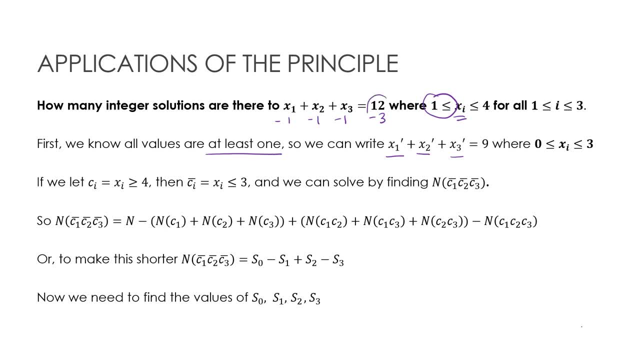 and x3 prime are now equal to 9, because 12 minus 3 is 9.. And notice, I've shifted this from 1 to 3.. Nope, I've shifted this from 1 to 4 down to 0 to 3.. I really like to have that 0 here. It makes 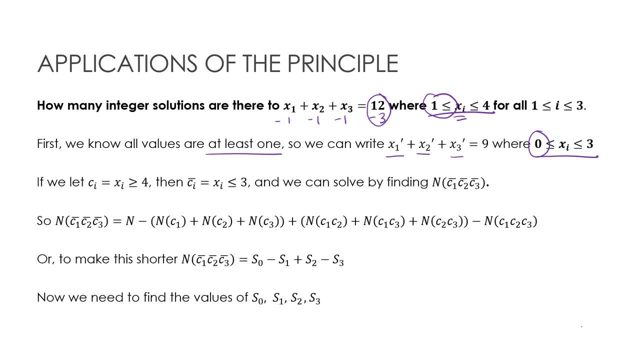 it a lot easier. Okay, now we're going to say we're going to let c1 be that xi is greater than or equal to 0. So we're going to say c1 is greater than or equal to 0. So we're going to say: 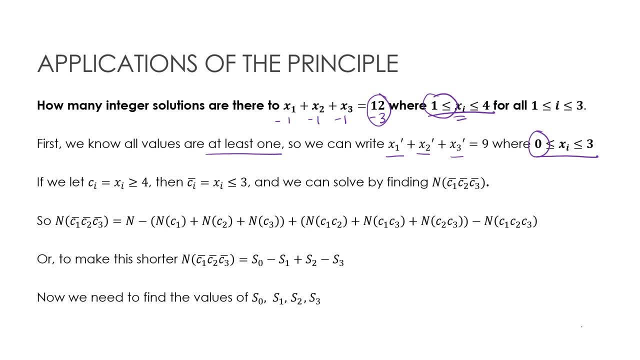 equal to 4.. So why am I doing that? Well, because I know that 4 is not okay. Remember, I'm saying I want to find this only works from 0 to 3.. So from 4 on to infinity, those aren't okay. So if 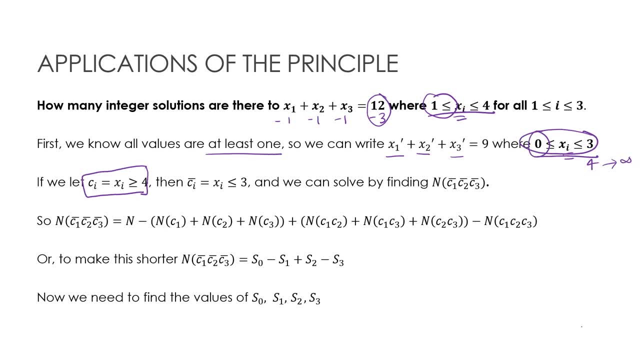 I set this condition to be greater than or equal to 4, then I'm really going to be looking for not ci, Not ci. I know how to find because we've just been working on finding not ci. So to solve this question, I'm really looking for not c1,, not c2,, not c3, because that's what I've set my conditions. 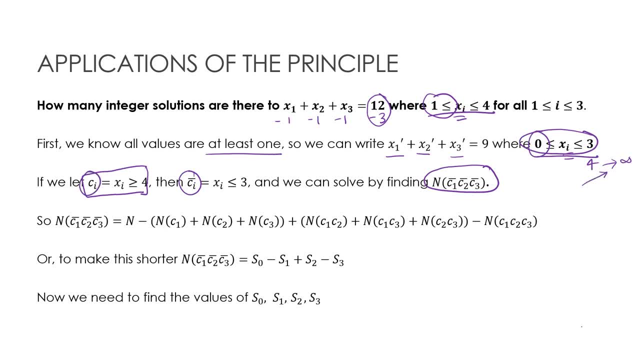 to be is that they're values outside of my range, So hopefully that makes sense. This is just a repeat of everything we know. that says: if you want to find not c1,, not c2,, not c3,, you take the universe, you subtract elements. 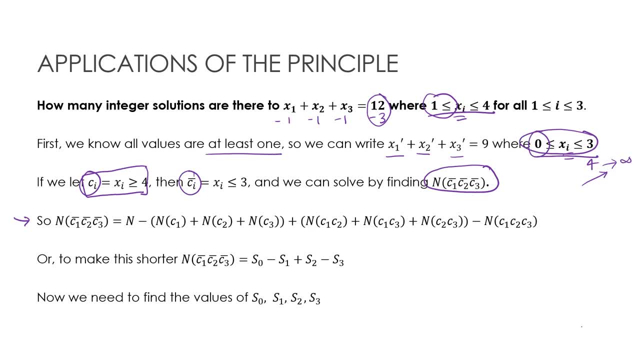 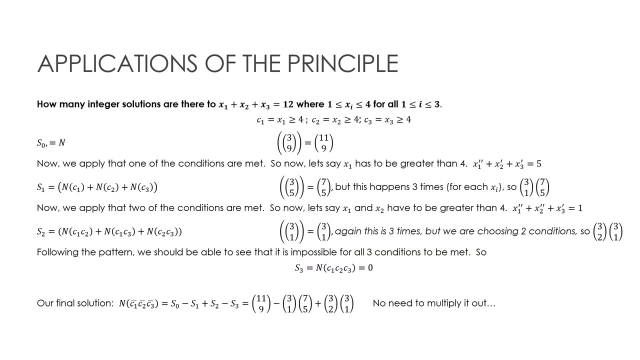 or the number of elements in set size 1, add set size 2, subtract set size 3,, etc. which may also end up looking like this: So really, all I have to do is find each of those four values. So our job. 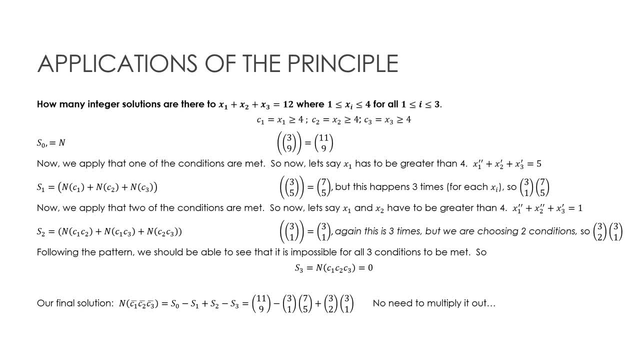 then is to find the values of s0,, s1,, s2, s3, etc. Now, s0 is just the number of elements in the universe, So really I'm starting to figure out how to find the values of s1, s2, s3, etc. So I'm 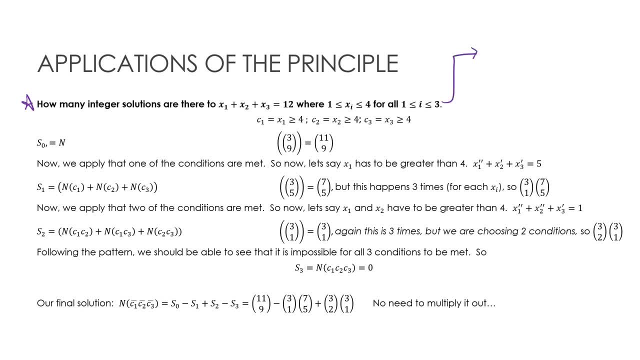 starting with this question, but remember that on the last page I rewrote this to say: x1 prime plus x2 prime plus x3 prime are equal to 9, because I used the fact that they were all at least 1.. Then I said, and of course I said that now 0 is less than or equal to x sub i is less than, or. 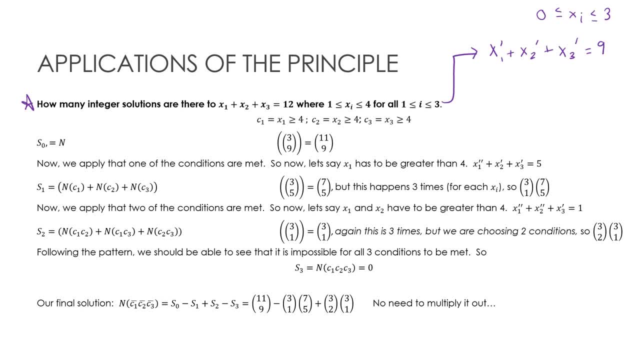 equal to 3.. Then I made my conditions: c1 is that x1 is greater than or equal to 4, because now it tells me I'm going to be looking for not c1.. c2 is that x2 is greater than or equal to 4,. c3 is that x3 is greater than or 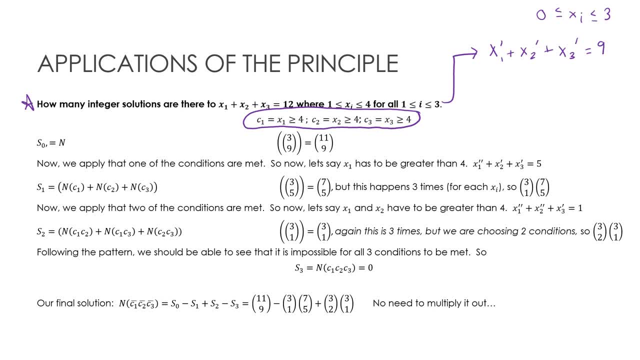 equal to 4.. So let's take a look now at kind of putting together the principle of inclusion, exclusion, as well as something that we've already talked about, which is combinations with repetition. What I'm saying is: now I have three boxes, And those three boxes 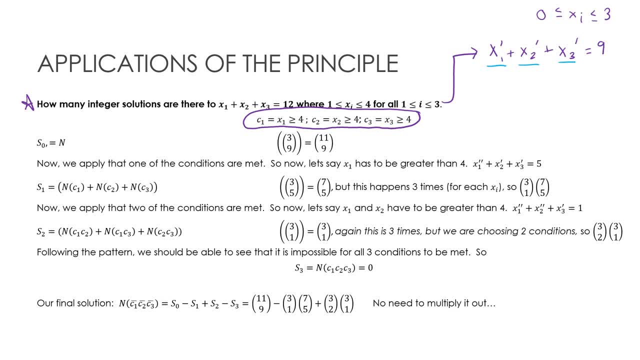 three boxes. the number of elements I put into each box have to add up to nine. So I have nine items to place. So I could place three and three and three. So that's one of the different ways I could do it. I could place two and two and five. That also adds to nine. So you get the idea that 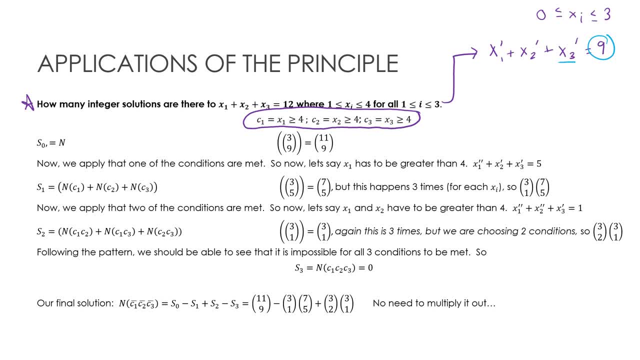 there are a lot of different combinations and I'm much too busy to come up with all of them. I just want what's the total number. So let's use combinations with repetition. that says I have three boxes. I have nine items to place, Remember. combinations with repetition says three choose. 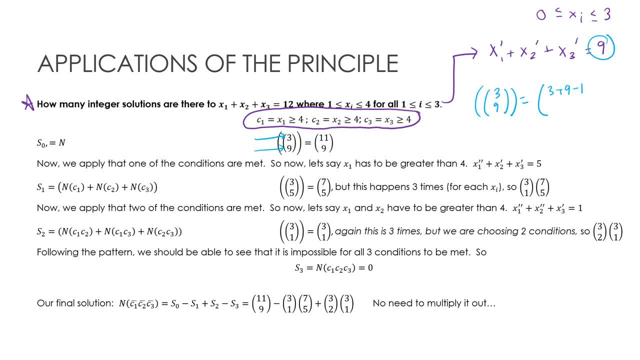 nine is three plus nine minus one, So I would subtract that one choose nine, and that's where eleven choose nine came from. Now, could I get my calculator out and determine what eleven choose nine is? Yes, you don't need to do that. So notice, in my final answer I'm including eleven choose. 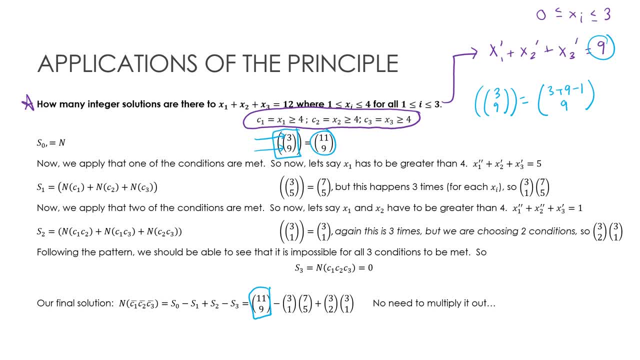 nine. I would not include combinations with repetition three choose nine, because I would want to write it as a normal binomial coefficient. Now we're going to apply that one condition is met, One condition only. So if one condition is met- essentially I'm saying c1 is met- Let me use a different color. 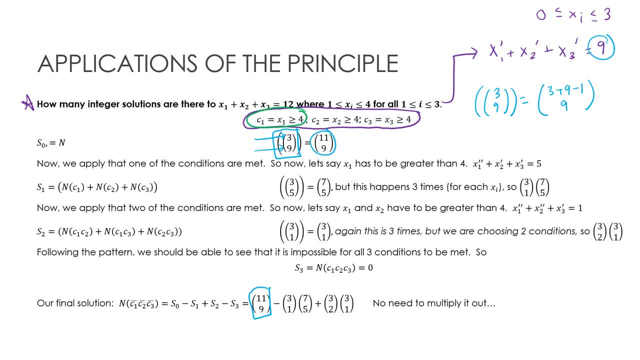 So I'm saying let's say c1 is met. Well, if c1 is met, then c1 is at least four. So I could do that. So I'm going to write it as a normal binomial coefficient. So I would take four away from here and here And that gives me that x1 double prime plus x2 prime. 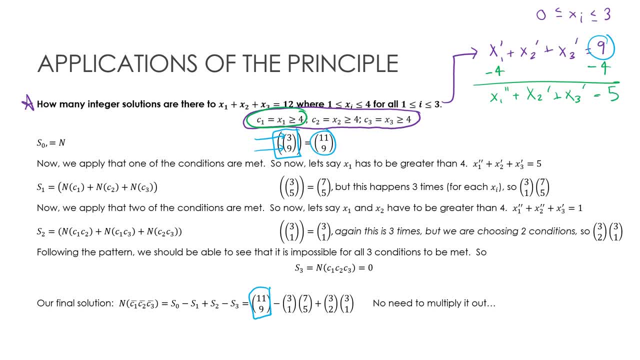 plus x3, prime is equal to five, Which means now I have three boxes and five items to place. Three items, three boxes, five items to place is three plus five, which is eight minus one is seven. Choose five, But it would happen for. 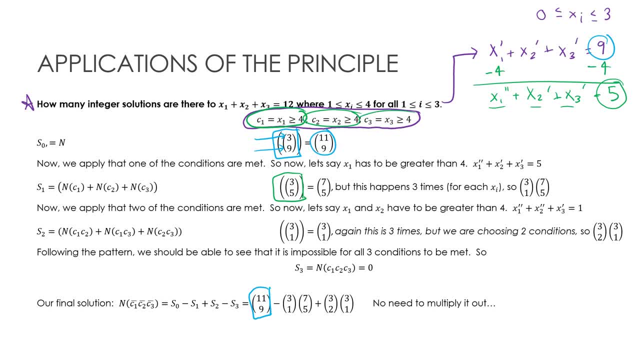 for x1, then for x2, then for x3. So how many times will it happen? It will happen. The seven choose five times three choose one, because it's three times one for each one. So I'm saying there are three conditions. One of the conditions is met. 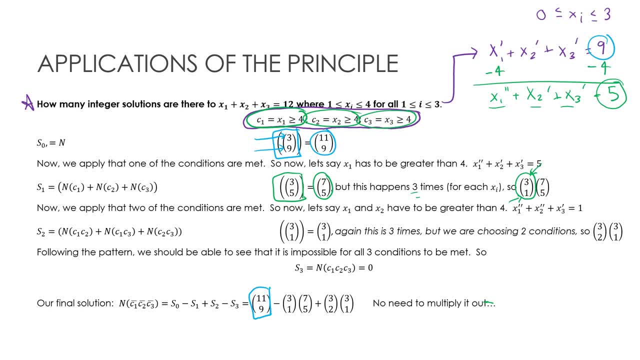 Then let's look at if two conditions are met. So if two conditions are met, I would say that four conditions are met. Now it's two and five there ceiling. so for this one regarding you should be four, three would you should be seven, maybe eight, If two conditions are met itself. 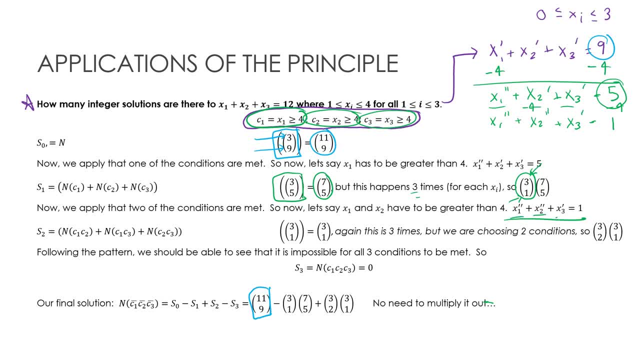 then you're saying: four items are met. Now let's make sure that those items are set. stop and take this into consideration. if I had to, let me find G1. nobody's going to satisfy me for that, So that's the final conclusion. Choose one Again. this is happening three times, but I'm choosing two conditions. So 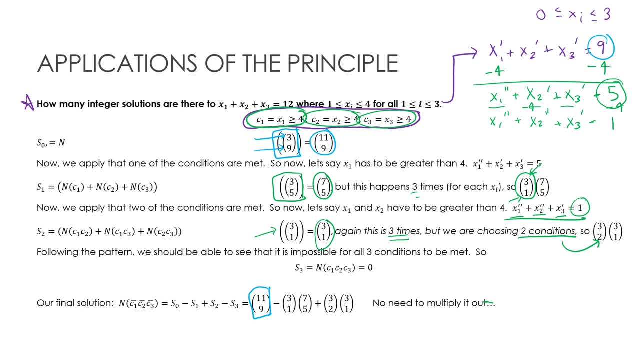 three conditions, choosing two of the conditions. Then if I tried to do that for all three, where all three are greater than four, we can see that if I subtracted four again, I would end up with a negative number. So it's very clear that S3. 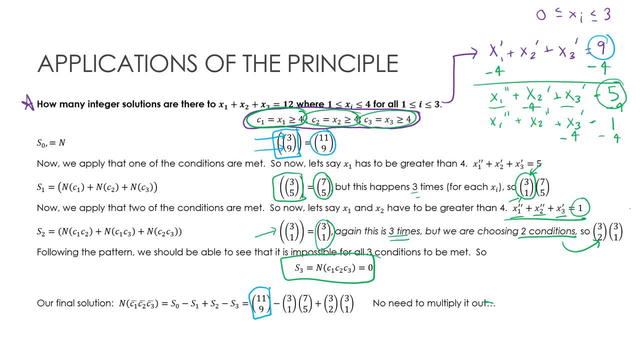 is actually zero, or the number of elements in the union of all three sets is zero. So what's my final solution? Again, notice that I did not find any of the actual values. I'm writing it just like this. I'm saying here's the number of elements in the universe. 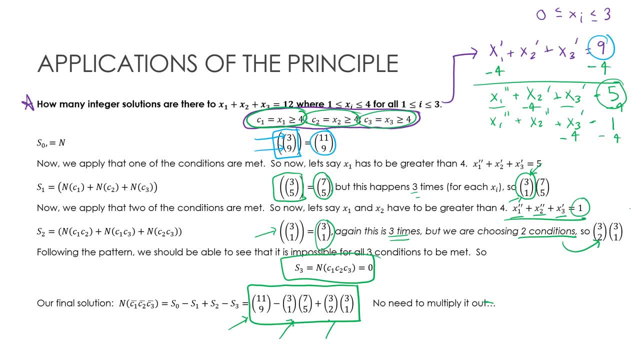 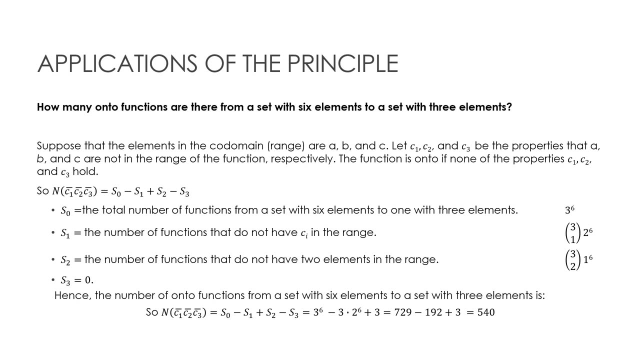 Here's the number of elements where one condition is met. Here's the number of elements where two conditions are met, And, of course, subtracting zero for when three conditions are met. That's my final solution. Okay, Let's take a look at another application of the principle: How many onto functions are? 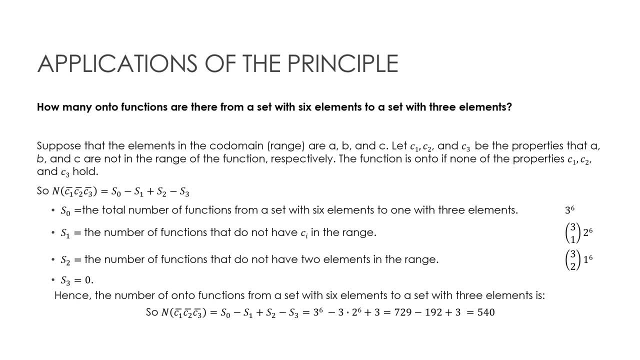 there from a set with six elements to a set with three elements. So remember that what I'm dealing with is: I've got six elements here And I've got three elements here And it says: let's let the codomain be ABC. So C1 is that A is not in the range, C2 is not in the range And C3 is not in. 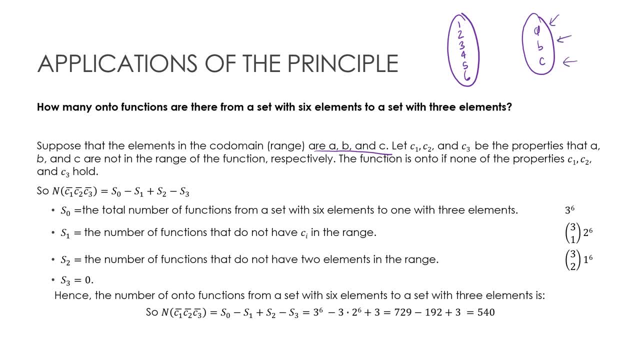 C2 is that B is not in the range and C3 is that C is not in the range So far. hopefully you're with me. So why did I say not in the range? Because my question is actually that they are in the range. so I want the not not in the range. 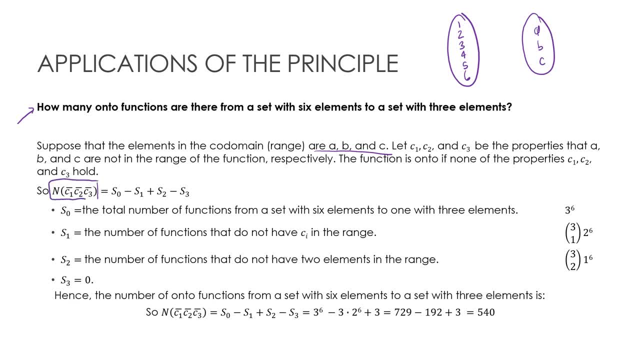 Get the idea. We always do the opposite so that I can then find not C1,, C2, C3, which means I get to use my handy-dandy little formula that we've been working with. So remember that onto functions are functions that each element in the range maps back to only one element in the domain. 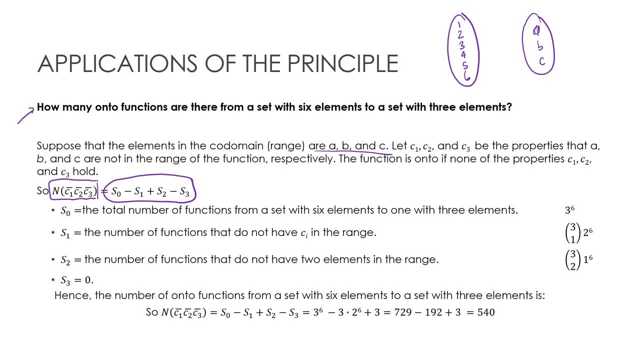 So first I'm looking for not an onto function, I'm just saying how many functions exist, from a set with six elements to one with three elements. So again, I'm looking from this direction. this guy can go back to six different values. 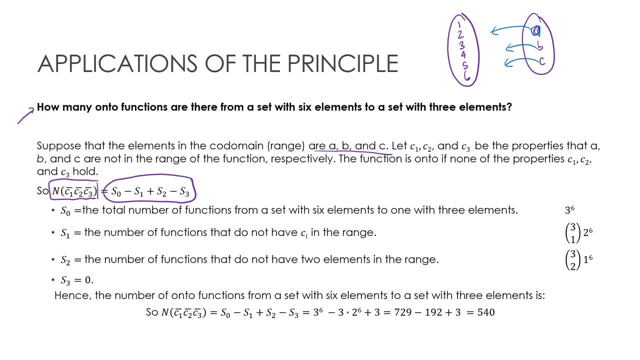 this guy can go back to six different values. and this guy can go back to six different values. So three values each to the sixth. Then I'm saying let's say C1 is true, C1 being that A is not in the range of the function. 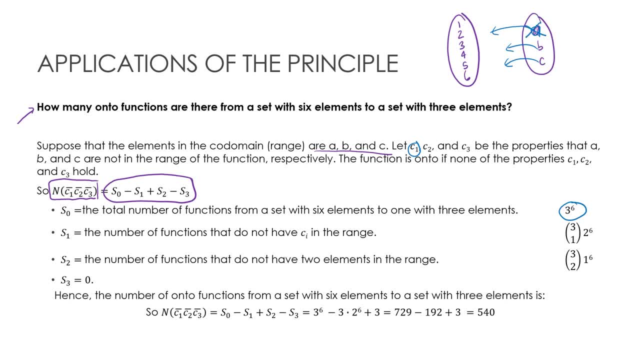 So if I took A out, I just have B and C. So now I have two elements, each with six options. But I have three conditions and I'm choosing one of them, Which means it's happening for C1, then it's happening again for C2, and then it's happening again for C3.. 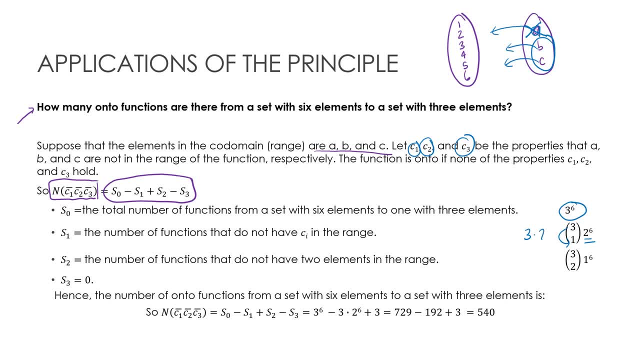 So basically, it's saying: we're taking three times two to the sixth is really what's happening? Then we're saying, let's let two conditions be true, Which means A and B are not in the range. Well then, I only have one guy to the sixth power. 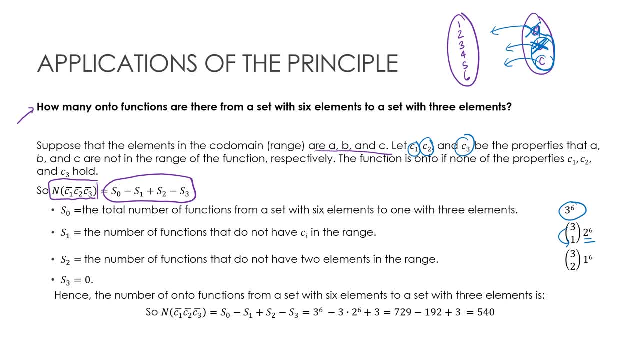 But that's. That's two conditions. There's three of them. Three. choose two conditions, which is the number of functions that don't have two elements in the range And then, of course, the number of elements that don't have three in the range would. 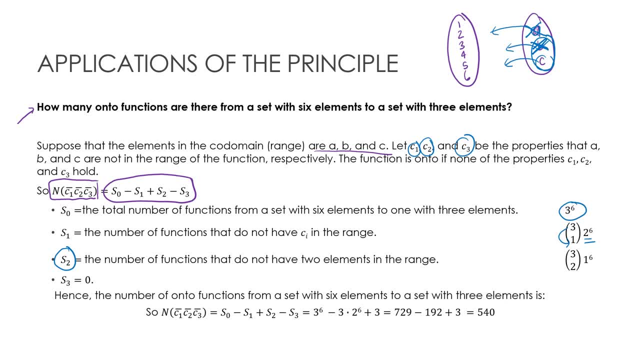 be zero, because that has to map to something. So, using this formula, I'm really just adding and subtracting the values that I need to Three to the sixth minus three times two to the sixth plus three times one, which is three. 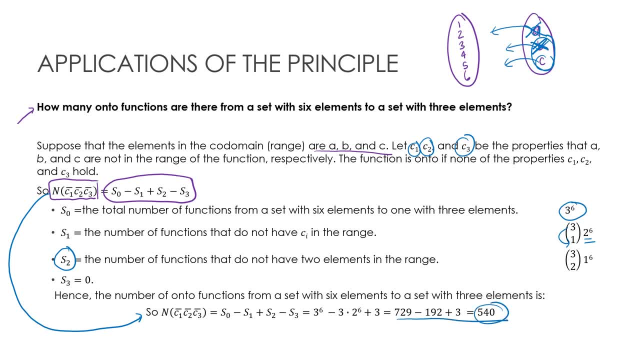 Which gives me 540 total. So notice, on this one I did go ahead and figure out the answer. Really, either one would do So if I kept it as three to the sixth minus three: choose one. two to the sixth plus three, choose two, one to the sixth. that would be just fine as well. 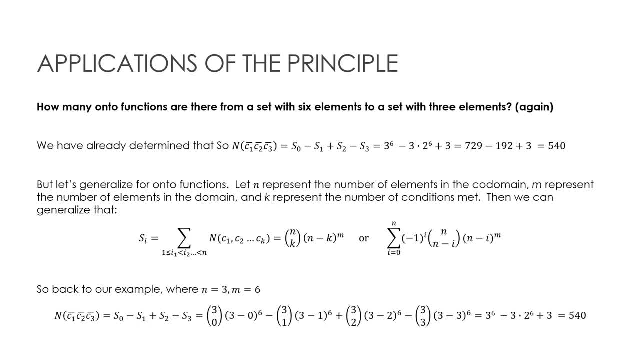 Now you're going to get a lot of questions dealing with onto functions. So just to generalize so that you have something to look back on. We already know that the answer is 540.. We've worked it out together. But let's take a look at a generalization of the function that says: hey, if you want. 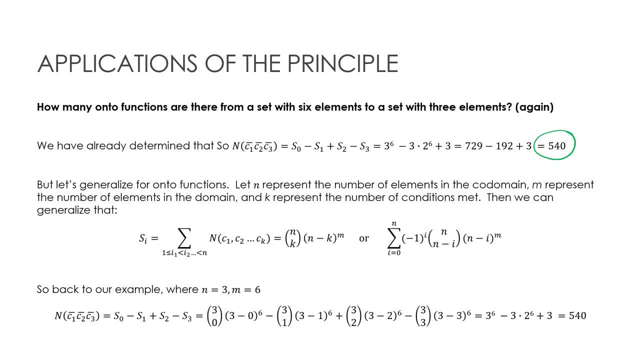 to find s sub i, so s sub zero, s sub one, et cetera. we're essentially going to find n, choose k, where n is the number of elements in the co-domain. Remember, co-domain is just range. m represent the number of elements in the domain. 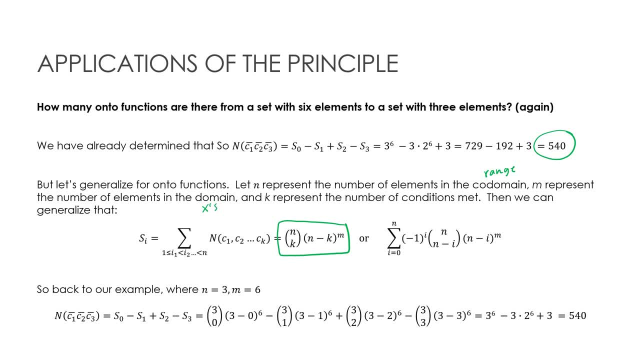 That's our x's, Here's our y's, And k is the number of elements in the domain And k represent the number of conditions met. Perfect, Then we can generalize essentially that each one looks like this. Or again you can use that summation notation with a negative one that helps you to remember that we're alternating between pluses and minuses. 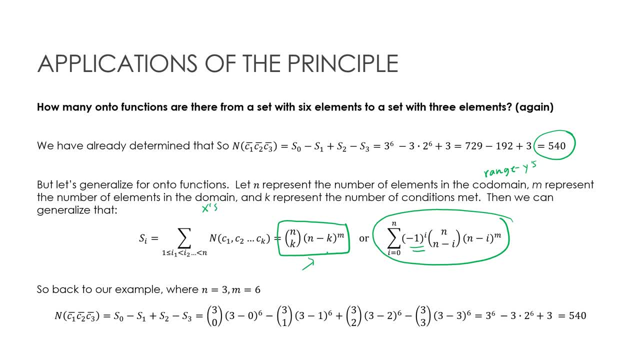 But essentially, if I'm using this, I'm saying three choose zero, because there are three conditions and zero of them are met, because that is s sub zero that I'm looking for. So in this case, n is three, k is zero. 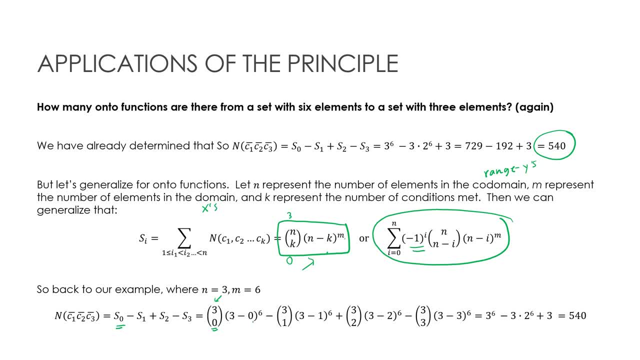 This would be three minus zero, And then m is the number of elements in the domain, which, remember, was six. So that's why I'm taking it to the sixth. That's what gives me three to the sixth, And then I move on to one. condition is met. 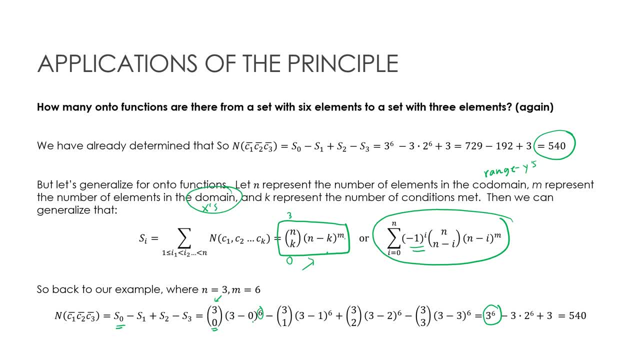 So I'm changing k from one or, sorry, from zero to one, But everything else is the same. So now I'm saying three choose one, And then three minus one to the sixth, And then I'm saying two conditions, So three choose two. 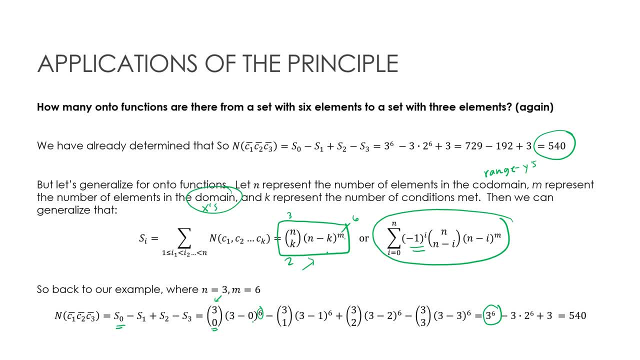 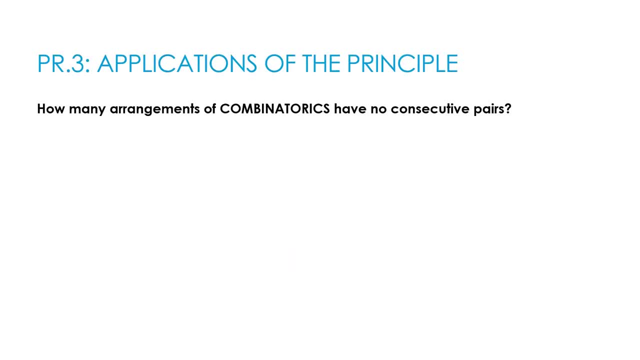 Three minus two to the sixth, And then three, choose three, Three minus three to the sixth, And notice, using that, I get the exact same answer as before. So I have two questions to finish this out, and they're both questions that I'd really like for you to try. 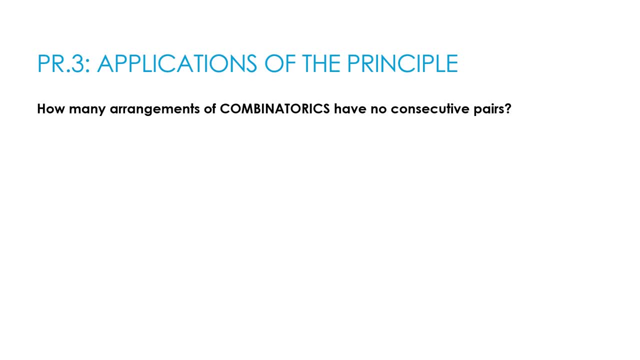 It really is helpful, even if you struggle with this, to get as far as you can on your own. before you press, play To see how I approach the problem. Also keep in mind there's more than one correct way to approach the problem. 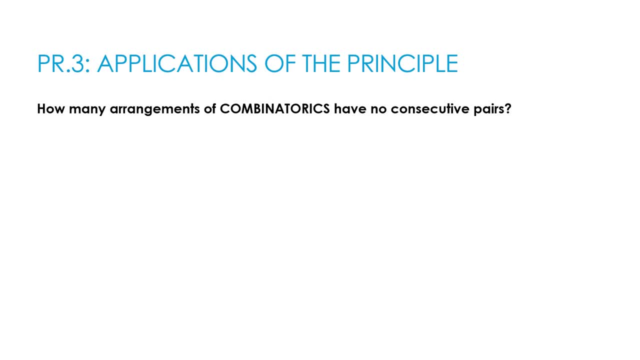 So I am going to go through this the way that makes most sense to me, But if you have a way to go through it again, we're still using the principle of inclusion-exclusion, So just make sure you're using that to solve this question. 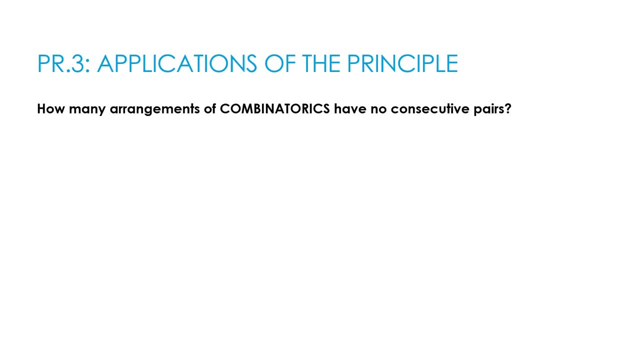 So this question says how many arrangements of combinatorics have no consecutive pairs. So before I do anything else, I would count the number of letters. And I've counted the number of letters total And there are thirteen letters. I also would want to remember that I've got some repeats of letters. 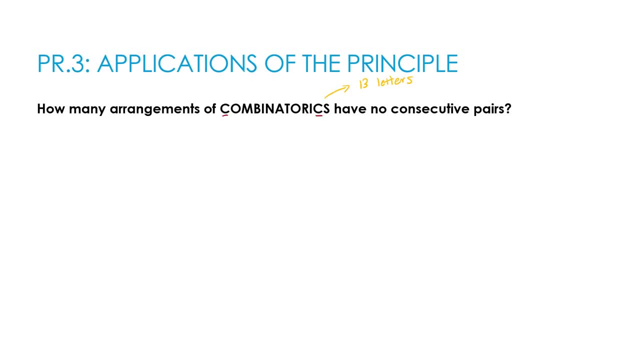 So, if you'll notice, I've got two C's, I've got two O's And I've got two I's, And all of the rest of my letters are singles, which is great. So why is it important to know what repeats I have? 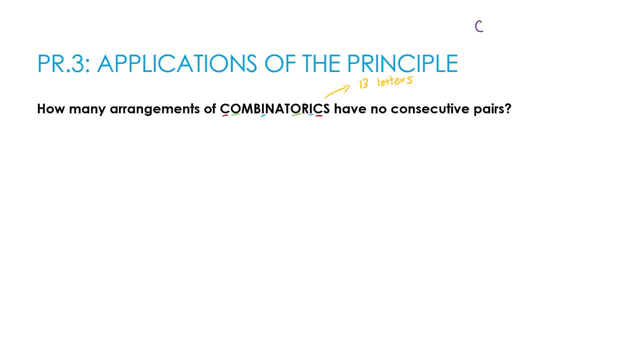 Because if I started to rearrange these and I had the two C's together and then C-O-M-B-I-N-A-T-O-R-I-S, this would be the same as if I switched these two around, because it's the exact same nonsensical word. 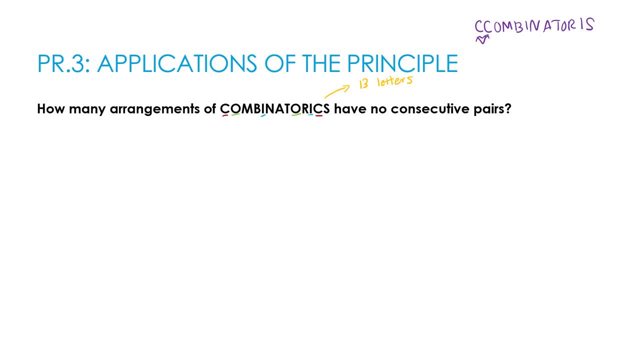 Still two C's together. So why do I bring that up? Because, if you'll recall, the first thing I want to do is find S sub zero, which is the number of elements in the universe. Well, if there are thirteen letters, the easy way is thirteen factorial. 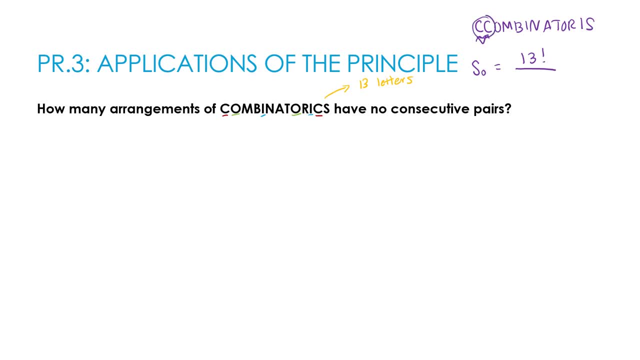 but it's not that easy because I've got the two C's that could end up together. I've got the two O's that could end up together and the two I's that could end up together. So that's the number in the universe. 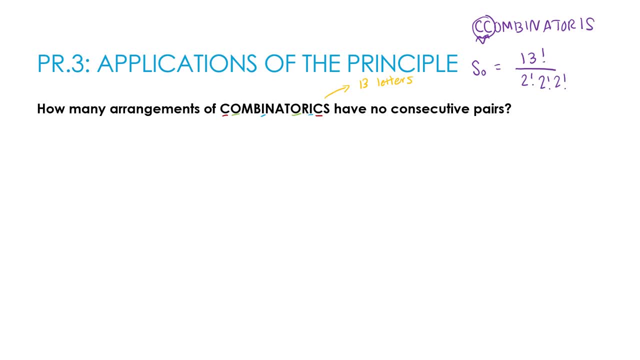 What would we do for our conditions? Well, our conditions if we want no consecutive pairs. that means when we write our conditions, we're saying we do have consecutive pairs, because we always do the opposite. so that when I'm finding my solution, 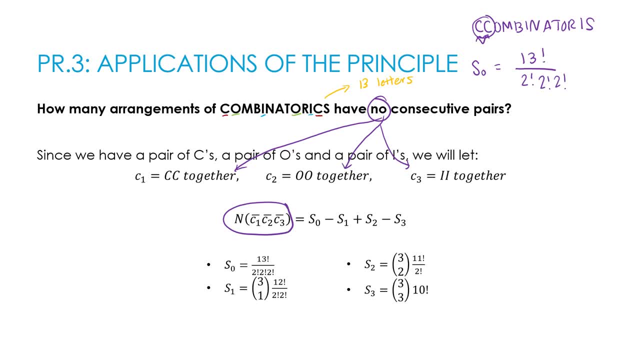 I'm finding the no consecutive pairs. So C-1 is that the two C's are together. C-2 is that the two O's are together. C-3 is that the two I's are together. So if I want to find S-1,. 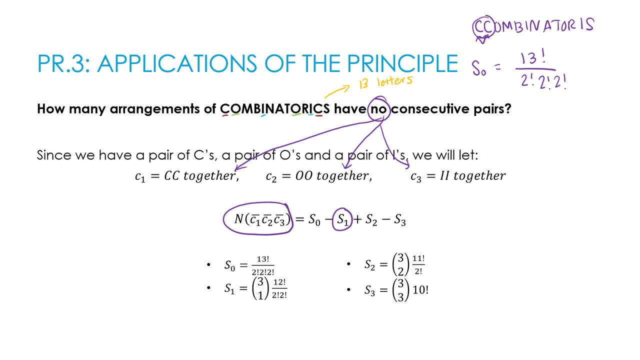 the number S-1 would be that one condition is met. So either the two C's are together, the two O's are together or the two I's are together. So how would I determine that? Well, it's going to kind of look like this: 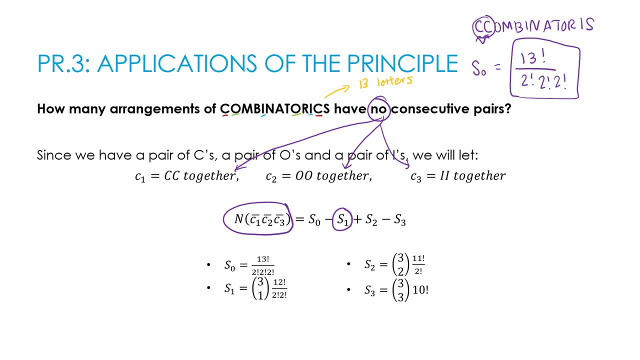 but what I'm going to think about is if the two C's are together, I'm just going to call that one letter. So the two C's are one letter, which means now, instead of thirteen letters, I have twelve letters. and how many pairs do I have? 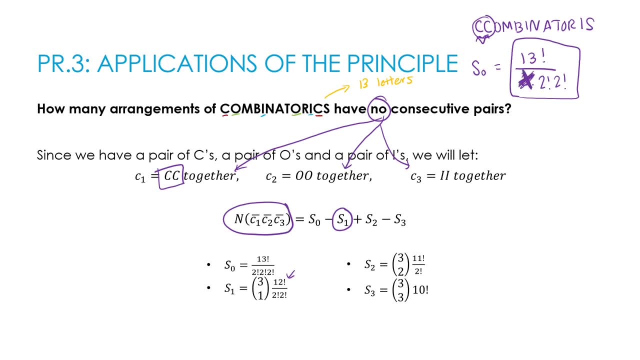 Well, I've already taken out a pair, because I've said those two C's are now just one letter. So now I've got the O's and the I's, So it's twelve divided by two factorial divided by two factorial. Why is it three? choose one. 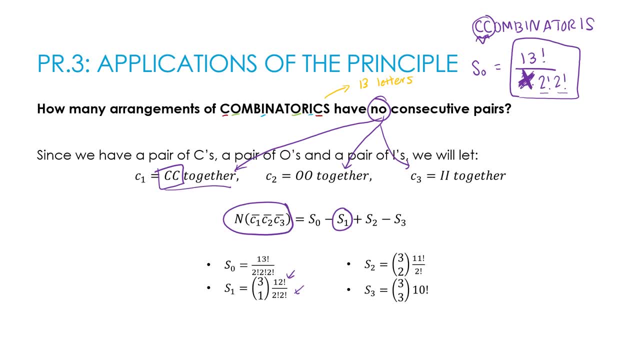 Because there are three conditions and I'm choosing: either that C-C is together, or that O-O is together, or that I-I are together. So that's S-1.. Then I'm going to do S-2, and S-2 says let's fuse the two C's. 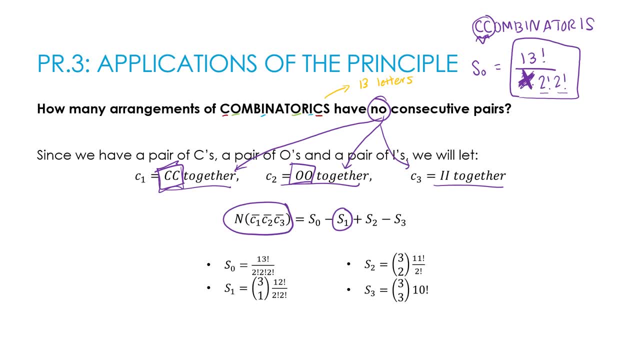 and fuse the two zeroes- I'm sorry- O's. So now I have eleven letters. I've got the two C's, I've got the two O's and then I have everything else, which means I have eleven letters and just one pair. 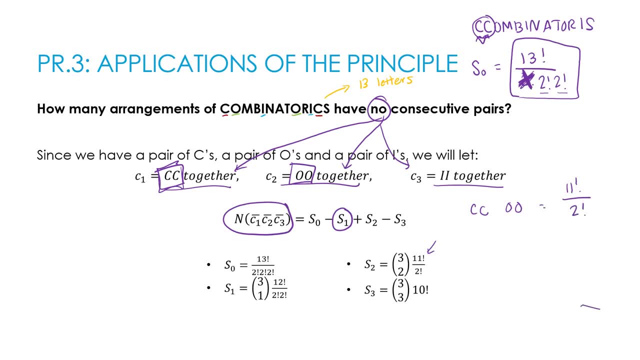 which is the I's in this case. Now, if I did the same for the two C's and the two I's, then that would be eleven factorial, two factorial, and then the two O's and the two I's, that would be eleven factorial, two factorial. 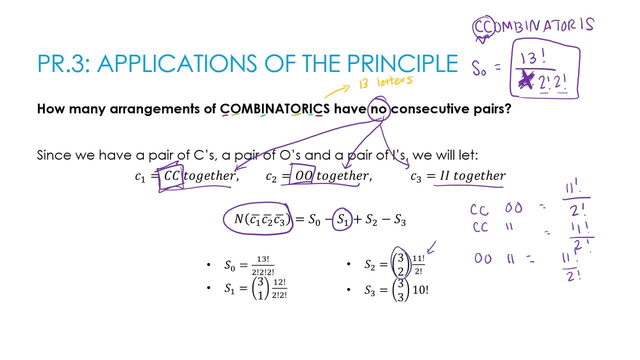 and again. that's why we choose that three choose two, because we're choosing two conditions. So it basically- so I don't have to keep writing eleven choose two that many times, Then we're going to say that all of them are together. 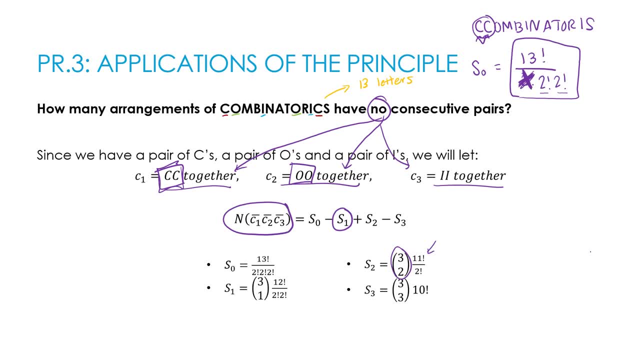 which means I've got one fewer letter because I've got CC together, OO together and II together. so now instead of thirteen letters I have ten letters. I don't have any repeats, so notice, I don't have to divide by anything. 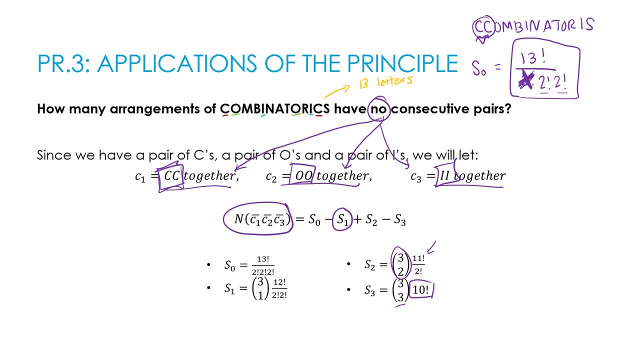 and there are three conditions and I'm choosing all three of them. So what's my final solution? I would just write it as thirteen factorial, two factorial, two factorial, two factorial minus three. choose one. twelve factorial, two factorial, two factorial. 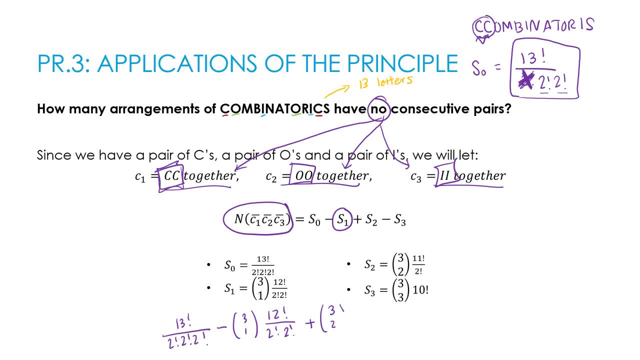 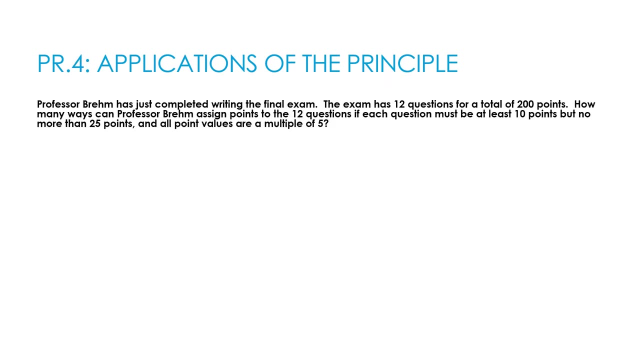 plus three, choose two eleven factorial. two factorial. minus three, choose three, ten factorial. That is my final solution. Here's your last practice question, and this one is a linear combinations question. So just to give you a start before I set you off on your own. 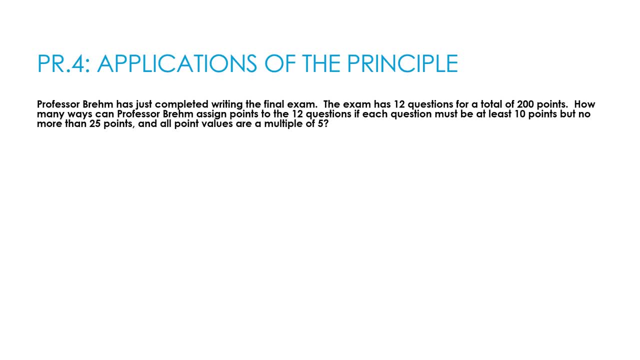 we did a question like this before, where we said: how many integer solutions are there for x1 plus x2 plus x3 equals twelve. Essentially, what I'm doing here is saying x1 plus x2 plus all the way up to x12, because there are twelve questions. 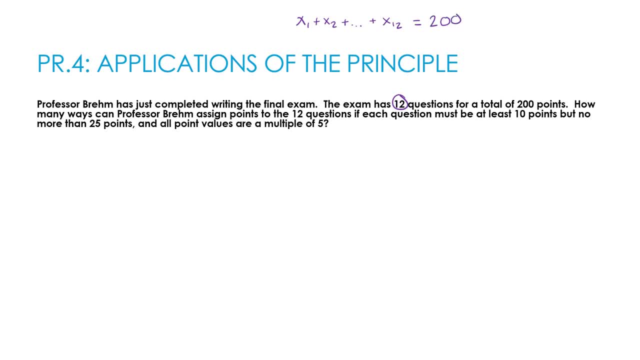 has to equal two hundred points. So you have two hundred points. on your final there are twelve questions. So how many ways can I assign the point values to the twelve questions if each question must be at least ten points but no more than twenty-five? 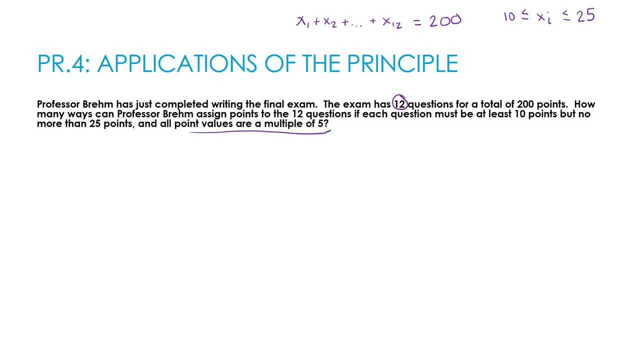 And all point values are a multiple of five. I'm going to let you figure that one out on your own. So think about how we could use the ten and the twenty-five like we did before, and then what would your conditions be? How are you going to solve this question? 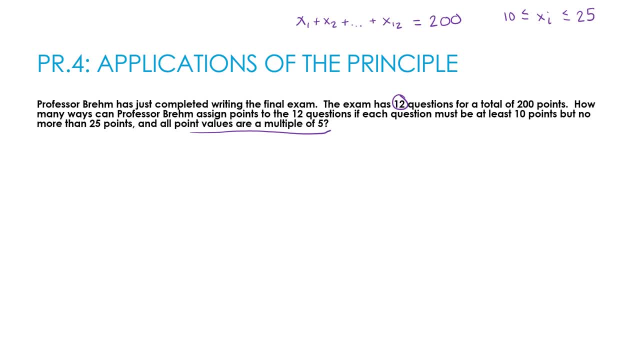 So really do press pause and take your time going through this. When you're all done, press play to see how you did, And if you did it correctly, then kudos to you, because this is a tough question. So again, first thing is exactly: 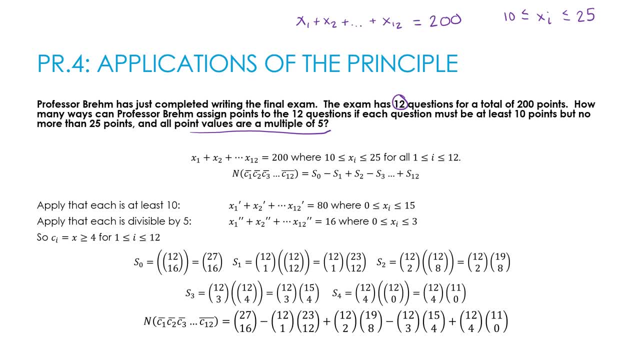 what I've already done with you. x1 through x12, the sum of those is two hundred. I've restricted them to be from ten to twenty-five. for all of the i's from one to twelve, which means just for every single question. 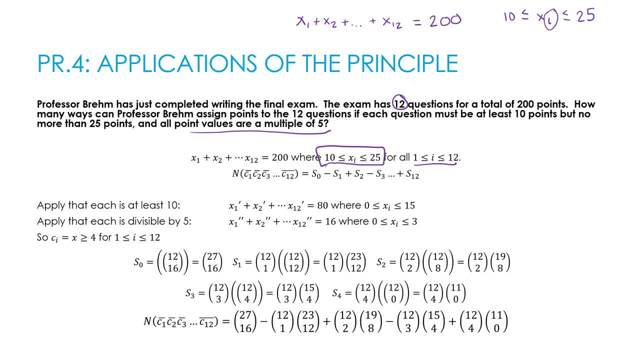 i being my subscript here. So I am going to first apply that each one must be at least ten. So I'm subtracting ten, subtracting ten, subtracting ten, etcetera from each one. So essentially I'm subtracting 120. 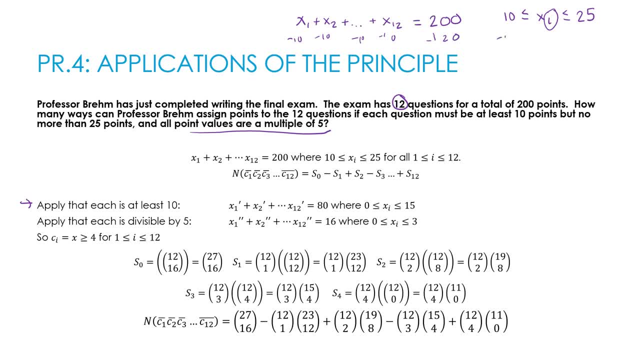 because there are twelve total. So again, that's going to give me now that my x prime values are between zero and fifteen. So x i prime are between zero and fifteen And that's really the first step. is you want to take that into account? 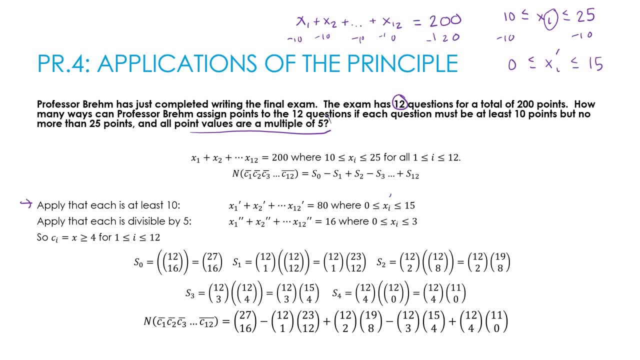 Then I'm going to apply in this case that all point values are a multiple of five. So if I'm dividing by five, then I'm getting x1 double prime, x2 double prime, etcetera, and then dividing eighty by five, 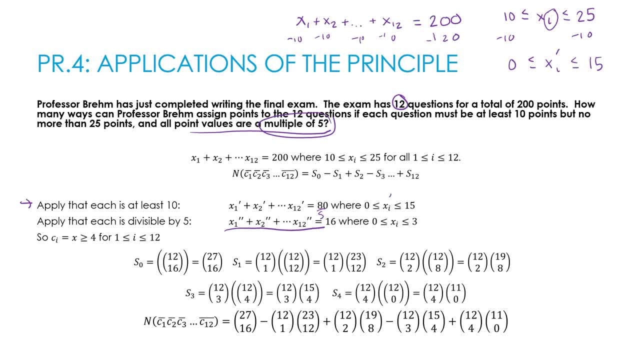 and that's where I get sixteen. And I divided this by five and this by five to say from zero to three. So now I've got it a little more straightened out. Now I'm going to look at the conditions. My conditions are that: c1. 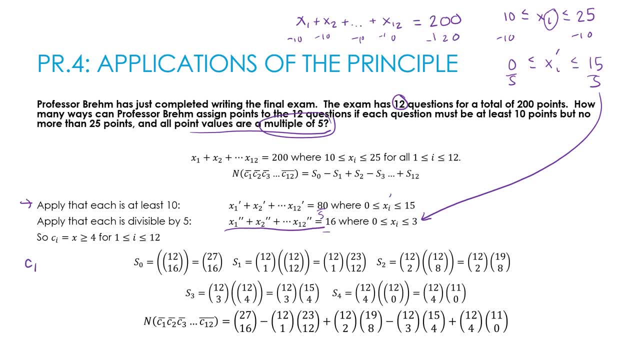 or ci. c1 would be that x1- forgot my i down there- x1 is greater than or equal to four, And then c2 is that x2 is greater than or equal to four. You get the idea. So there's twelve conditions. 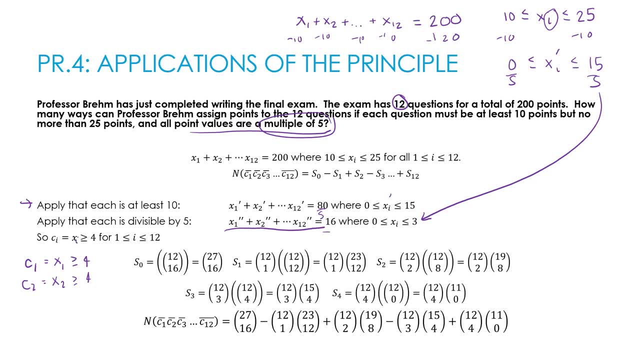 for just a single twelve conditions, because there's twelve questions To find the universe. I'm saying: I have twelve boxes, I have sixteen items. So combinations with repetition twelve choose sixteen gives me twelve plus sixteen minus one or twenty-seven. 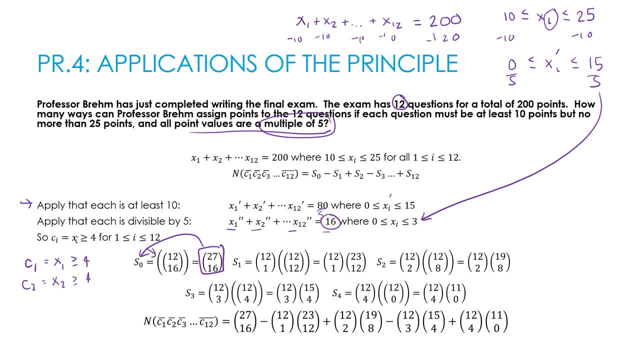 choose sixteen. that's my universe. S1 would be that I'm applying that four. So now I'm going to subtract four and subtract four, and now I have combinations with repetition: twelve, choose twelve, and that gives me twenty-three: choose twelve. 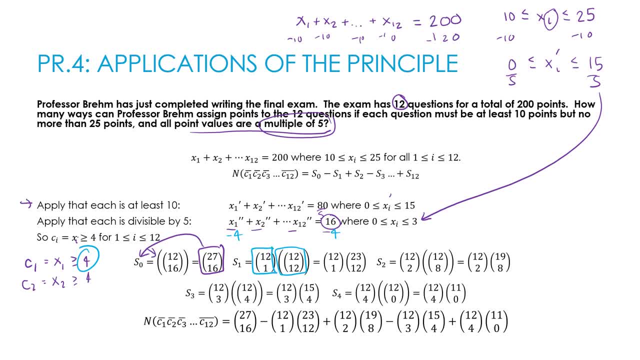 How many times is that happening? Well, there are twelve conditions, and I'm just choosing one at a time. So this is all S1.. Continuing on to S2, S2 would be that two conditions are met. So again now I'm going to subtract another four.